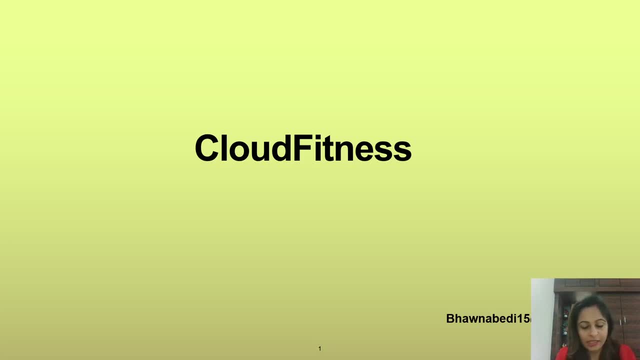 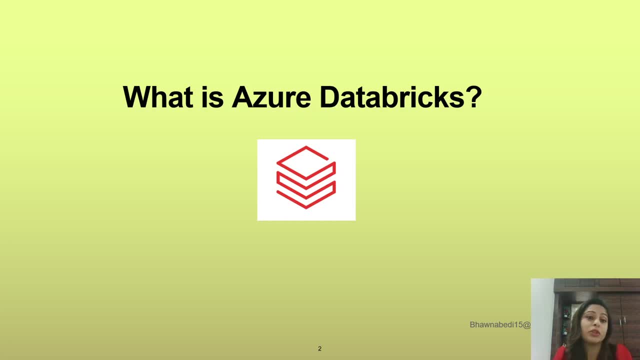 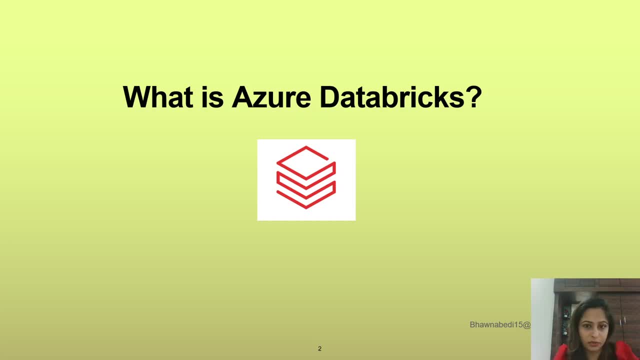 these 30 videos. I'll try to keep only important parts of it, not anything more than what is required, right. so now let's move ahead to what exactly is as your Databricks, but do remember to Like, subscribe and share my channel. so, essentially, this as your Databricks is a concept which is an extension to the map. 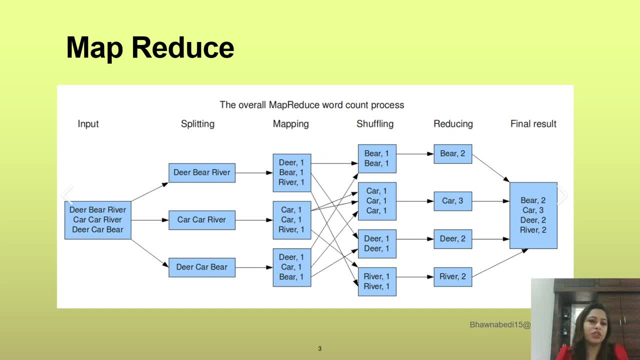 reduce concept. so if you want to really be strong at the app, you know at the basics of Azure Databricks, you should understand this map reduce concept. so this map reduce concepts were, you know, started by, was started by a Google in their research papers. I think in 2003 there was a research paper where they 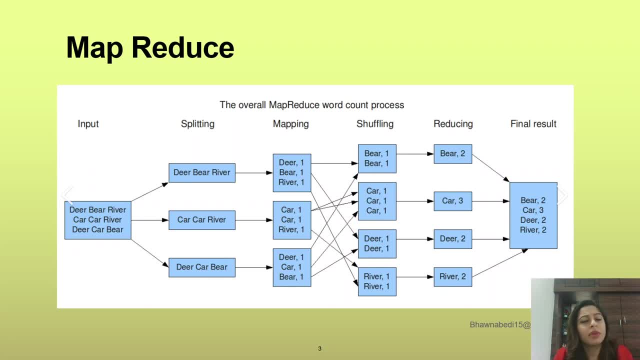 you know, had this concept of map reduce, but do remember, this map reduce was not in memory computation. I will explain this map reduce to you. if you look at the screen right now, what you see, I have just, you know, captured this from Google images. now, if you see here, 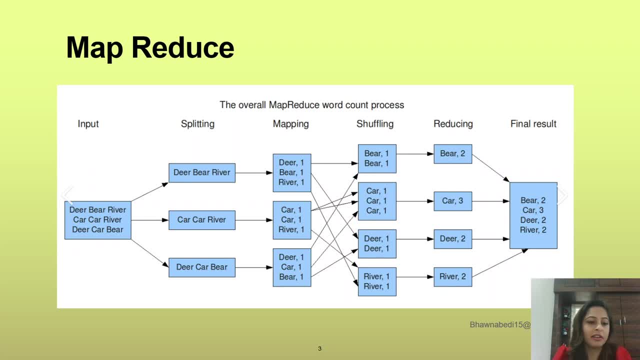 you have an input where you have deer beer River car car River deer car beer. so these are the different words that you have now in map reduce. you actually have to do a transformation on this input and essentially in the final output you need to count the number of deer, the count of each word. so let's say: deer how many? 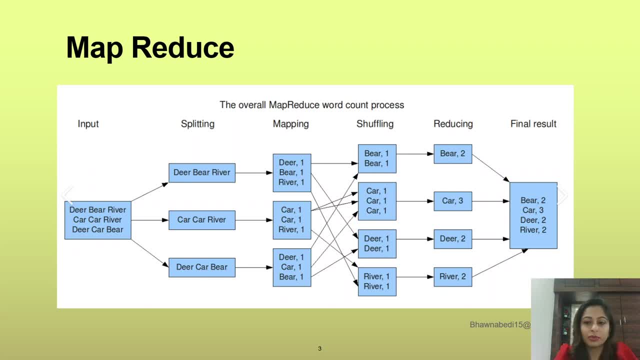 times this deer has come in this input it has come two times right. so if you see in the output you have deer comma two, car has come. let's say three times count of car has three. so this is essentially the count that you are doing on the data now. this is your input and that is the final output. now, essentially, 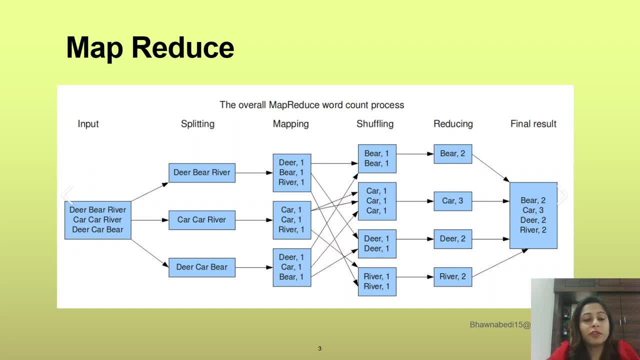 you have to do a transformation. so in this concept of map reduce, what we do is we split the data. so let's say you have a big file. so, since I'm explaining map reduce to you through this image, we have taken a subset of data right, a very 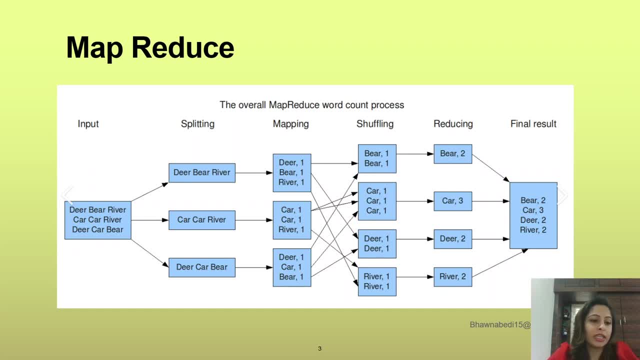 small data. but essentially, just imagine you have, let's say, one terabyte of data and you have to do, you know, this kind of count operation on it. so the point is to it right. this map, what does map reduce? you know the first stage of this map. 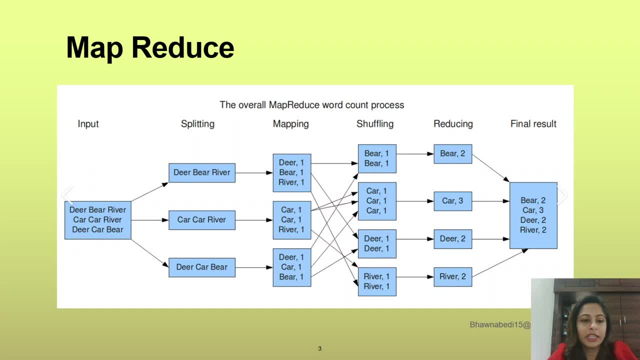 reduce. what it says is: you split the data. you know you have one terabyte, just split it. you know. so if you see it has three lines of data, right, so it has split the data. it has split the input into three rows and this you know: splitted output. essentially it will go to a different computer for the 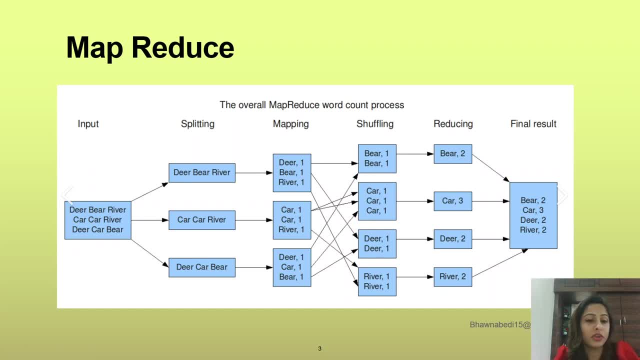 execution right, it will go to a different computer all together for the execution in parallel. so that is the concept of map reduce. so the moment you split the data you will be able to do computation parallely in different computers right in different hardwares. you will be able to do it now for each. 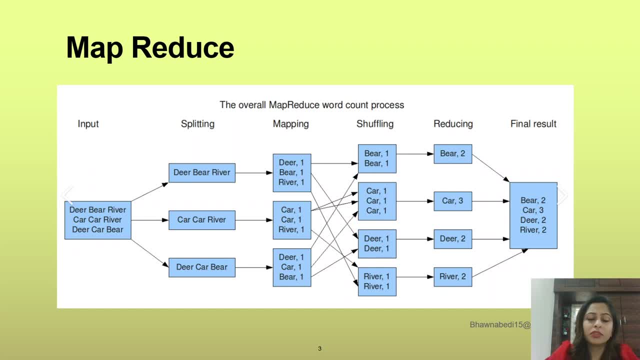 of these computers where you send this one input line, it will try to do the computation. it will try to do the mapping. mapping as in: it will see that in the first row you have dear one time. you have beer one time. you have river one time. so it is. 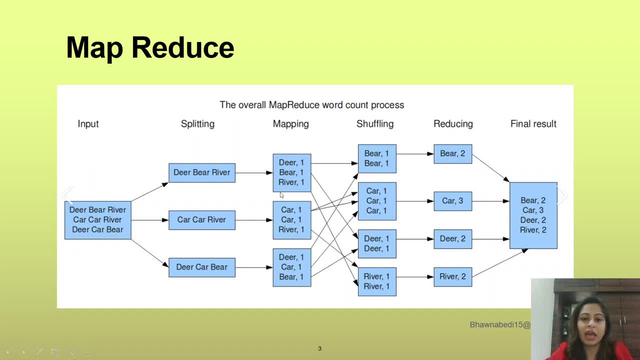 mapped to one, one and one. so each of the computer has mapped your data into the second stage, which is the mapping. now, once your mapping is done, data from all the computer is taken. and now, the moment you take the data from all the computers, you basically aggregate or you reduce the data, right? so reduce this, this part. 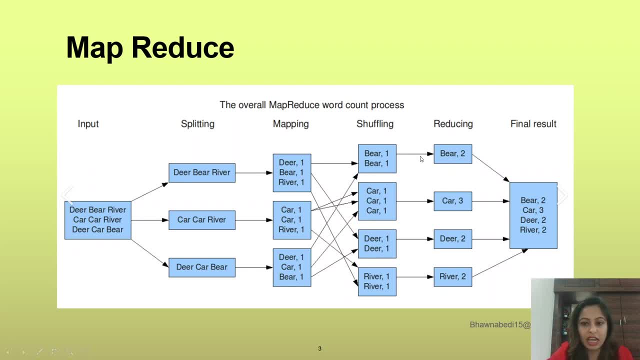 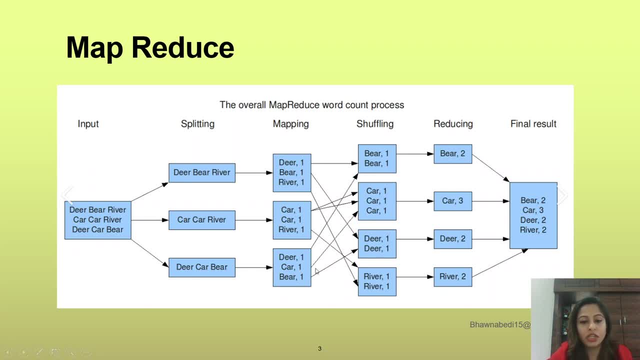 you need to take the data from all of these computers and then you need to combine that data. so you need to see that, yes, in the first computer is telling us that dear has come one time, and the third computer is telling us that the dear has come one time, so, total, the aggregated result, will be dear has. 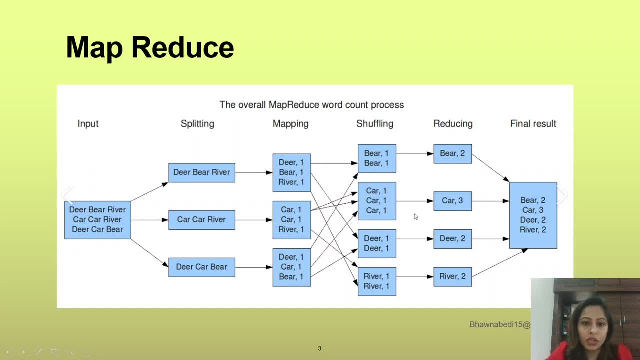 come two times right now. in this case, in this case, what you need to do is you need to check. you know each and every computer. you need to shuffle the data between each and every computer to check how many times beer has come- this is the- how many times car has come, how many times deer has come, how many times river has come. so this: 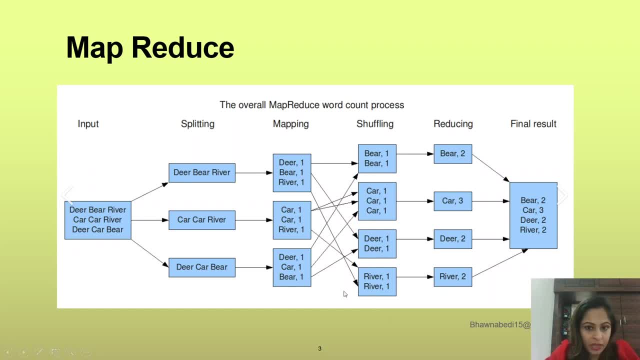 part is actually what is called as shuffling right. so this aggregation part and, uh, the the part which is trying to aggregate the data together, which is trying to get the data together and which is trying to get the count together, will cause shuffling of data between these computers and 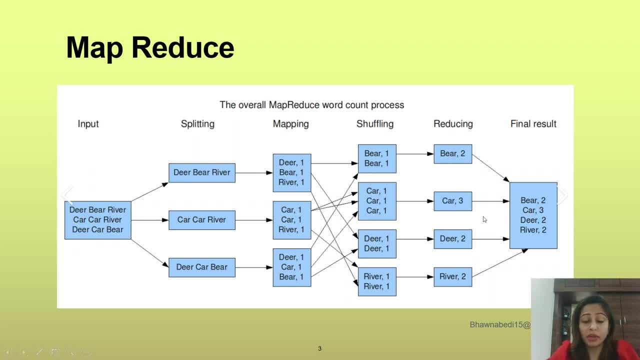 it will try to give you the final result. so this is the concept of map reduce. but the problem here is the basic problem, because it was done not in memory, it was not an in-memory concept so since it was not in memory, it became really very difficult to manage this data across multiple 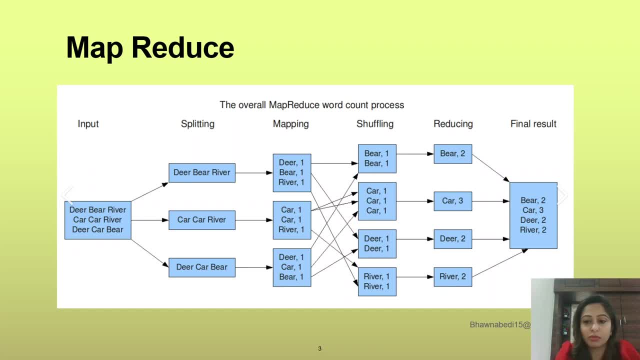 hardwares right across multiple small hardwares across multiple small computers. so now this map reduce actually turned into something that you know today as spark. so spark also does also similar kind of execution, but it does it in memory. so that is the basic problem: because it was done not in memory, it was not an in-memory concept. 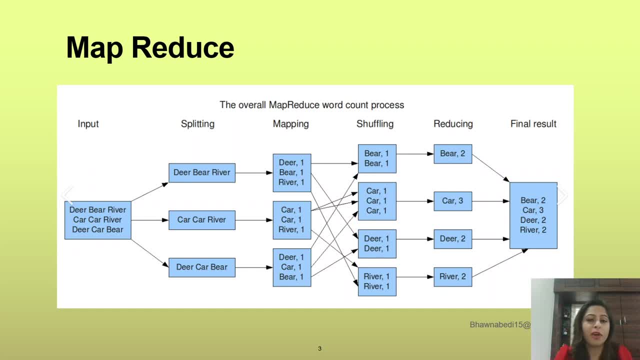 why, you know, in my previous video i have been talking about that spark is an in-memory computation. because all of this computation, what does this? this is essentially transforming the data. it is basically computing the data right. so this is called an in-memory computation, which is done. 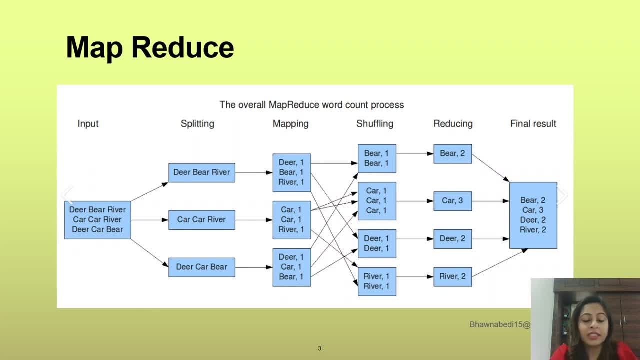 in spark now. so this was a background from where this data brick started. so now this map reduce was developed by you know- uh, i don't remember the exact name of the person, if i'm not wrong, mattie. so in his papers he basically developed this: you know, spark concept of in-memory computation and 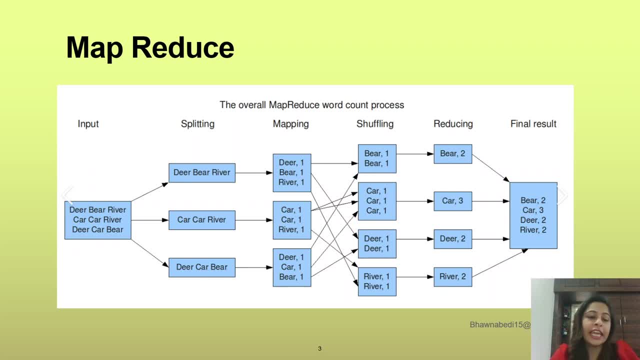 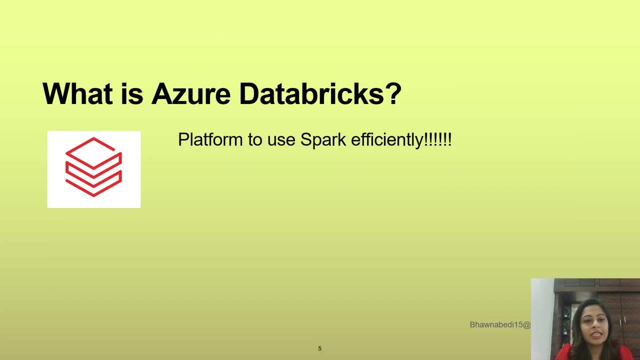 then he sold it off to apache spark and then they together built a company known as data bricks, right? so basically, the creator of spark itself has built data bricks. so now if you see what exactly is data bricks? data bricks is a platform where you can use spark, and now spark is created. 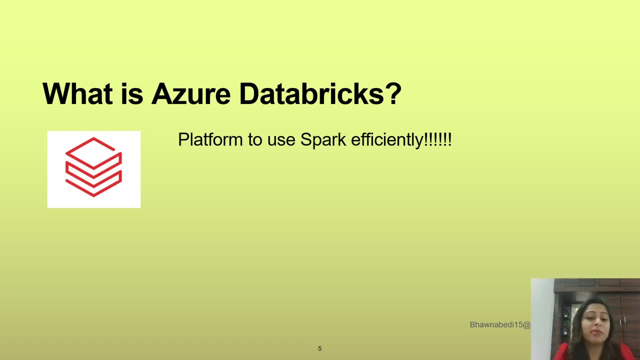 you can use data bricks and you can use data bricks and you can use data bricks and you can use recruit data and so on. so you have, because in that platform you you have map reduce earlier, which was doing not in memory computation. now you have spark, which is an in-memory computation of uh you. 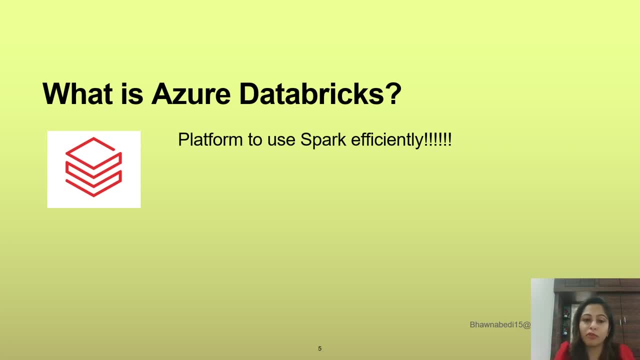 know big data basically. so you have a huge loads of data in different formats. now to do in memory. computation of that data? uh, you have a platform named as data bricks. it is a very simple definition, right you can. you know google and you'll have a lot of different definitions of azure data. 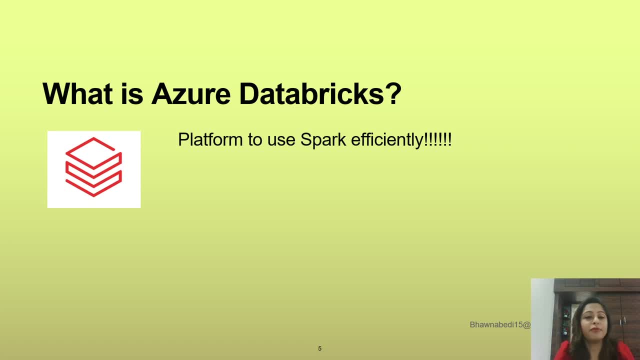 bricks. but essentially, the main definition is this: it is a platform to use spark right and now, since it is a platform, it is a developing platform. they have lots, of you know, optimizations over it, so you can use spark very efficiently in azure databricks. now coming on to the spark. 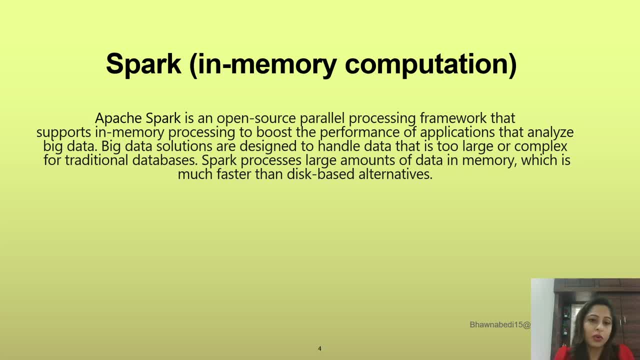 again. i'll go back one step to talk about spark. so, as i've already explained, spark is an in-memory computation. so now let us go through a formal definition of spark as well. so apache, spark is an open source parallel processing framework. now, when i say open source parallel processing, 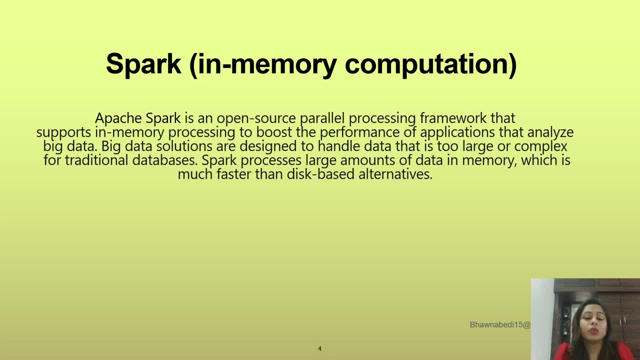 framework. it is open source, it is available to all. you can do a parallel processing, as i've shown, you know, in the map reduce. it follows the same concept, but in-memory computation. now it also, you know, since it is splitting the data into multiple in-memory machines right now, what 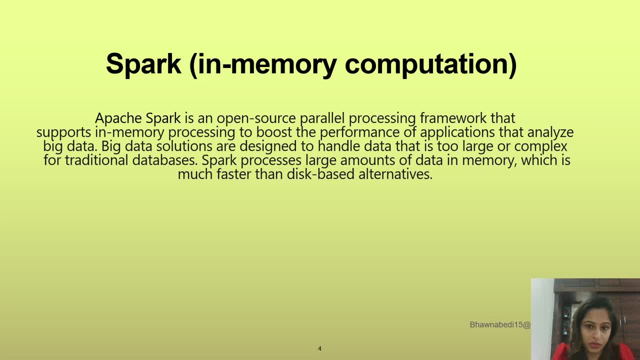 happens is it is able to perform parallel processing. so that is why you we are calling it a spark. so now let us go back to the first part of the video and let us go back to the parallel processing framework that supports in-memory processing to boost the performance. 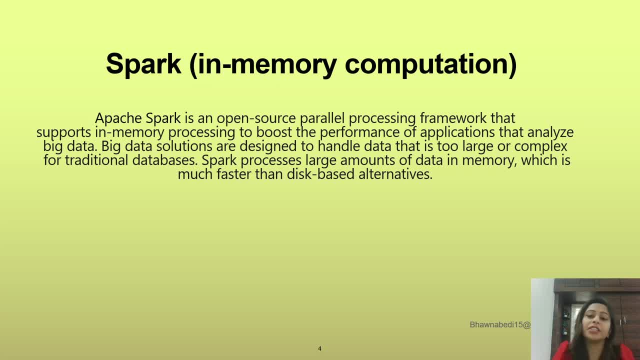 of applications. now, since it is in-memory competition, it is definitely much more effective than our map reduce, which was actually performed on the hardware. it was actually performed on the computers. now it is definitely used to analyze big data. so here you get the first definition. apache spark is an open source parallel processing framework. that supposed that. 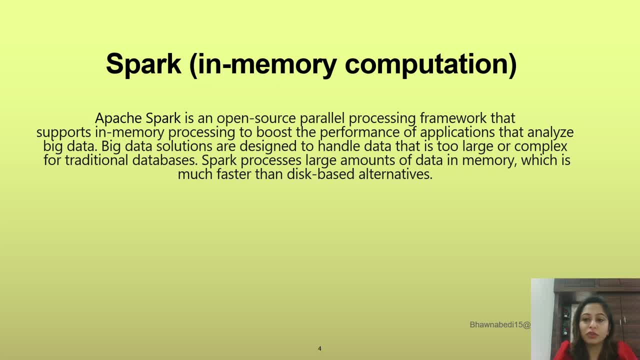 supports in-memory processing to boost the performance of applications. now, since it is an open source parallel processing framework that supports in-memory processing to boost the performance of applications that analyze big data. right now, big data solutions are designed to handle data that is too large or complex for traditional databases. so, if you talk about you, 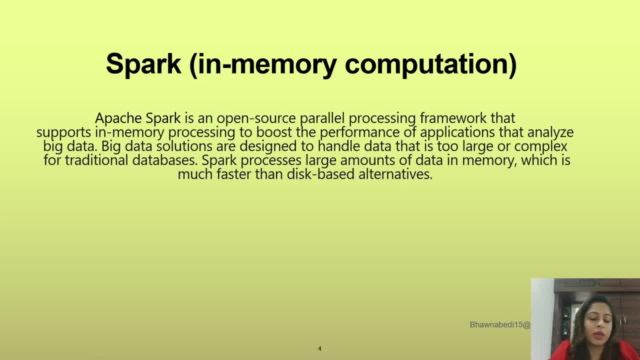 know traditional databases. you know you have structured data. you cannot process big data. you know big data. when i say big data, it has different formats as well, right? so traditional databases cannot handle your semi-structured or unstructured formats and they also cannot handle such a large volume of data, right? so spark can actually do that and similarly spark. 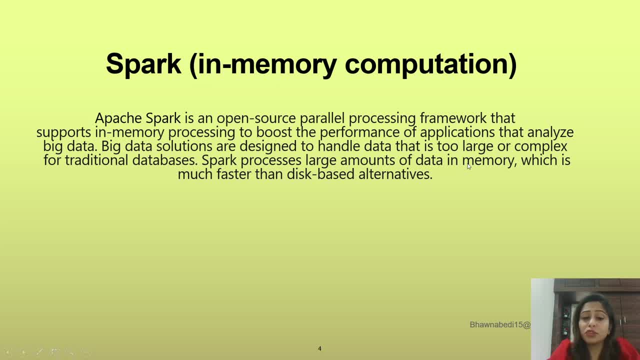 processes large amount of data in memory, which is much, much faster than the disk based alternatives. now, what is the disk-based alternative? is that map reduce. map reduces a disk-based alternative. so this is what your spark is, and data breaks is essentially only a platform where you can work in. 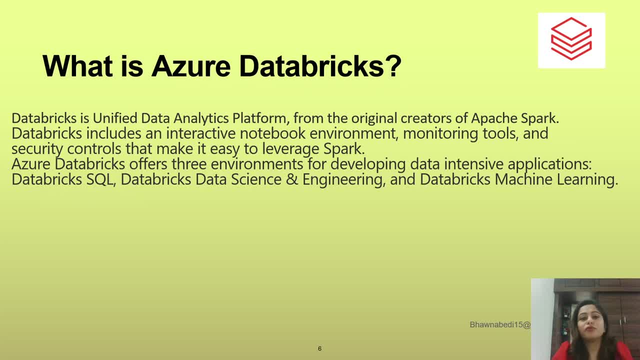 spark. right now, coming on to the formal definition of azure databricks, spark is a platform where you can work in spark. right now, coming on to the formal definition of azure databricks. spark is essentially So. if you see, Databricks is a unified data analytics platform. 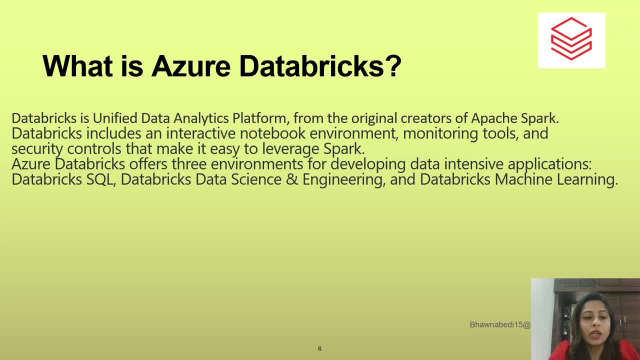 Unified data analytics platform. what does this keyword mean? So this means this? essentially means that this is a one place where multiple people can come together. When I say multiple people can come together, if you see, data analysts can also work in Azure Databricks. 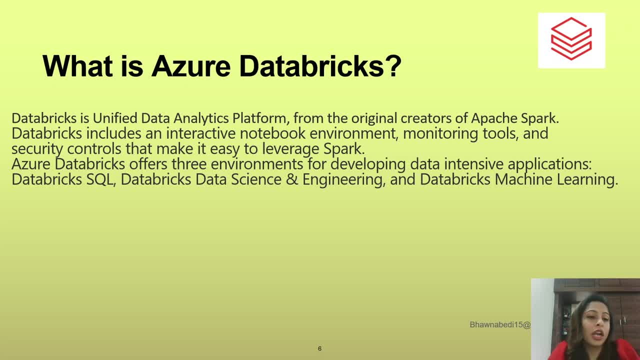 Data engineers can also work in Azure Databricks. Your data science and machine learning team can also work in Databricks. So that is why it says unified data analytics platform. You can analyze the data together in a single platform. right, And it is from the original creators of Spark. 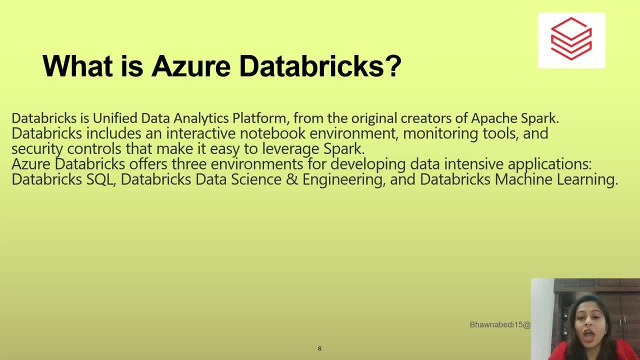 So, as I already told you, there was a person named as Matty who actually developed. I don't know if I'm pronouncing his name correct or not, but yeah, So he was the one who created Apache Spark and then he sold it to. he's the person who created this concept of you know, in memory computation. 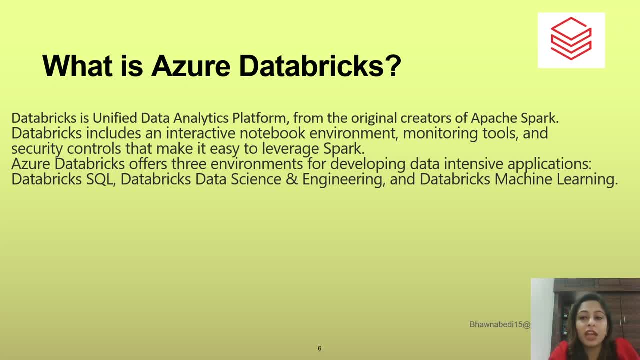 Spark, And then he sold it to Apache Spark and he developed this organization named as Databricks, along with the creators of. that is why you have this named as from original creators of Apache Spark. Now, Databricks includes interactive notebook environment. Now you know when I move forward with this series. I'll show you each and everything in detail. 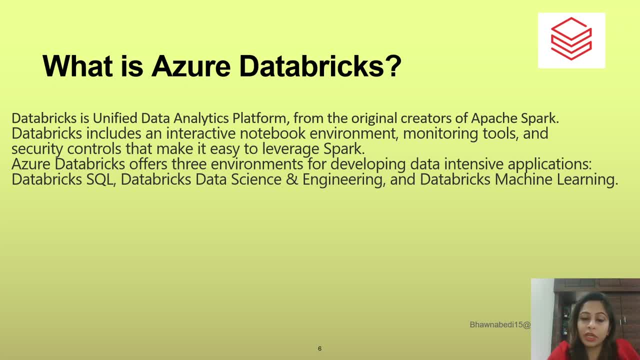 Now, when you talk about this, Databricks includes interactive notebook environment. Now, what you see is so. for example, You know you have to write a Spark, right? You? you have to process big data, So you need an environment, right. 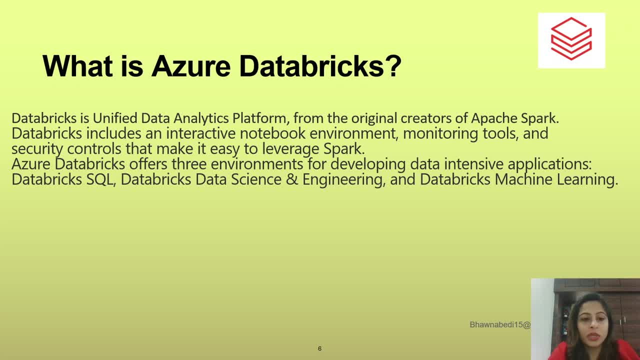 To write some code. So you need an environment to play with the data. So that environment is essentially called as notebook inside Databricks, So where you write the data. So if you have been, if you're familiar with Jupiter, so similar to the Jupiter notebook, you have something called as Databricks notebook where you can play around with the data. 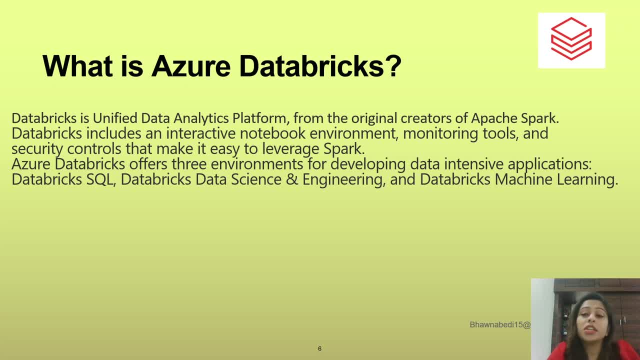 So it includes an interactive notebook environment monitoring tools. So it includes an interactive notebook environment monitoring tools. Now, once you create a job, basically if you come from any XYZ background, so let's say you have been working on any XYZ platform. 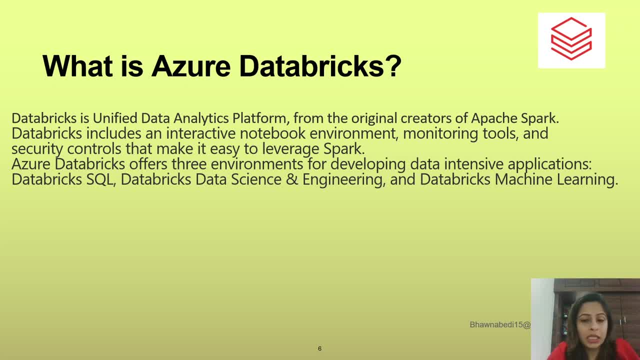 So there you create a job. you, let's say, you create a Python notebook itself. Now there also, you schedule it right. So you need a monitoring tool for that. Similarly, Databricks also has a monitoring tool inside it, which we will. you know. monitoring UI is the correct term. 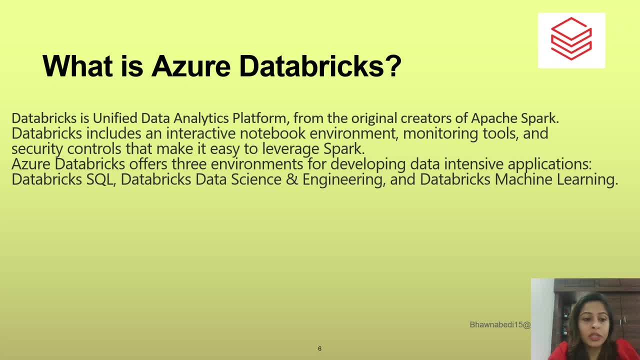 So it has a monitoring UI which we will see in the future videos, And then it has security controls. So definitely it is much secure. We will talk about this later on because otherwise it will become a very long video and that makes it easy to leverage Spark. 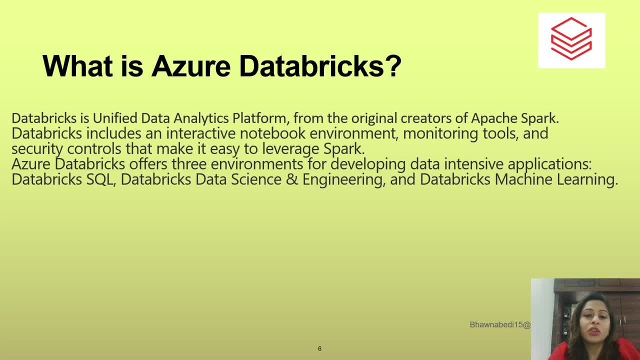 So why I am explaining each and every word to you is that you know. if you understand each and every keyword, well then, in that case you don't need to remember these. you know how do I say these, these kind of definitions, basically. 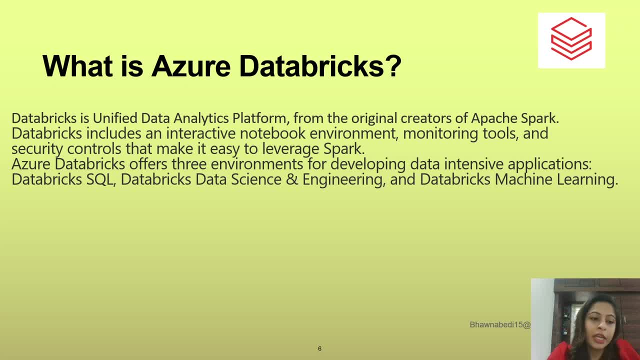 It will automatically. it should naturally come to you right? So Databricks offers three environments for developing data intensive application: Databricks, SQL Databricks, data science and engineering Databricks, machine learning. So inside Databricks you have three parts: Databricks SQL, which is essentially used by data analysts. much. then you have data science and engineering, which is used for you know your data science folks as well as your data engineers. 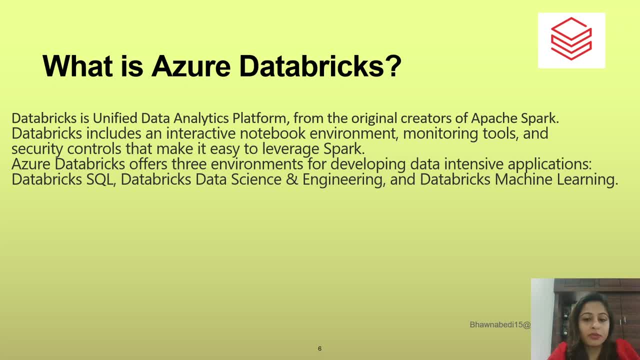 And then you have something called as ML, Databricks for ML, where you can train your models. So these are the three environments within Azure Databricks which we will actually see. the moment you see it, you will recognize it, you know much better. 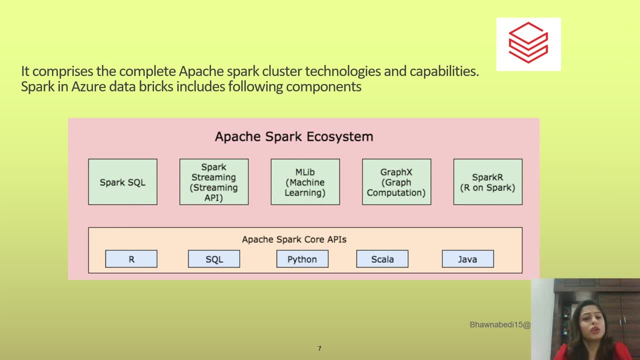 So now, apart from this, you know, since we have talked about Spark a bit, so I'll just give you a very small, you know, intro about Apache Spark, For example, this Apache Spark: right, It has multiple APIs. 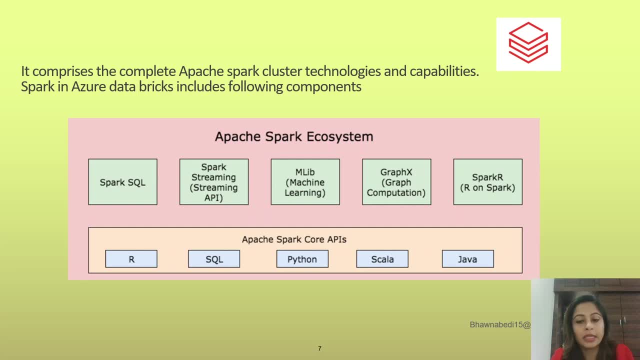 So the core APIs are basically R SQL, Python, Scala and Java. So the core APIs are basically R SQL, Python, Scala and Java. So in this, especially in the Databricks environment, you can write your code, since you have these APIs available. 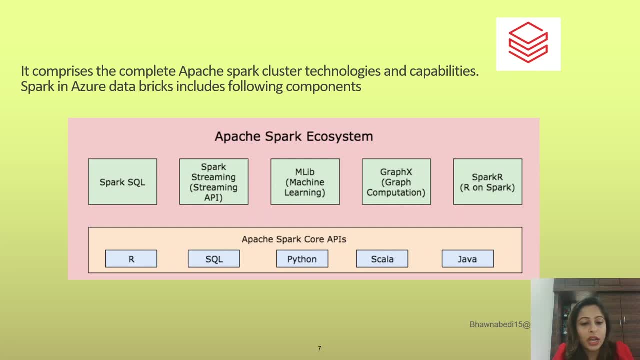 So if you write your code in R language, if you write code in the SQL language, if you write code in Python or if you write code in Scala, you can do that just because these APIs are available. So if you come from any of these backgrounds, it will become very easy for you to work in Databricks. 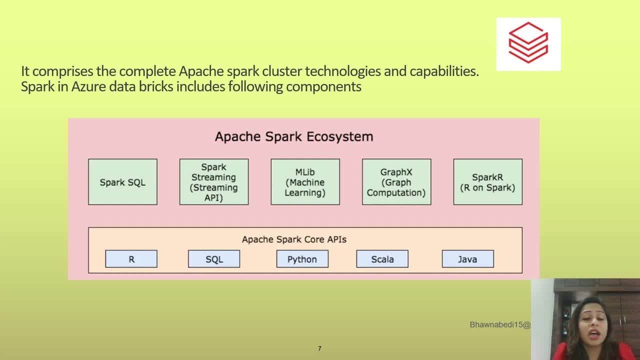 Similarly, it has, you know, APIs for the Spark streaming as well. So we will talk about Spark in a bit. Okay, talk about streaming uh in the little end of uh. you know this play series because streaming uh, streaming concept. i will talk about much in detail after we have covered the batch mode. so if you 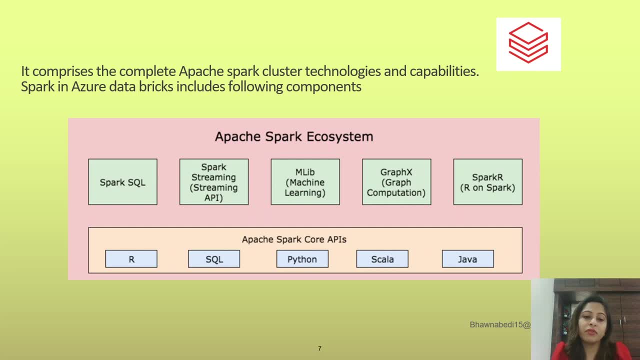 have data and you are processing it in batches. you are taking chunks of data and you are processing it in streaming. what happens is, as soon as the data arrives, as soon as the event arrives, as soon as the record arrives, you need to process it. so that is called a streaming. so apache spark has a. 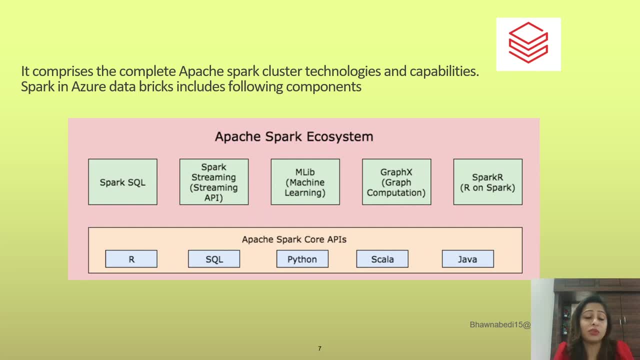 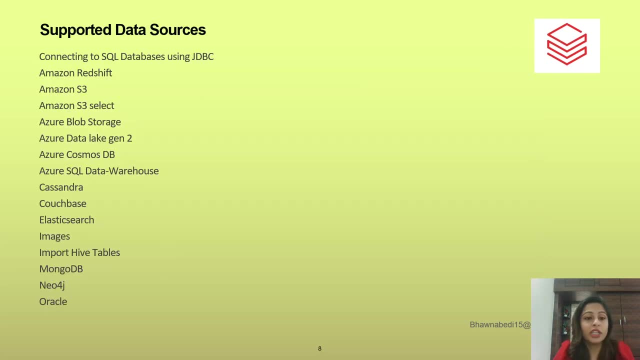 streaming api as well. it has a machine learning api as well. you can do graph computations as well. so it is a very, you know, big concept, and we are going to talk about even apache spark in detail. so coming up on to the supported data types, so when i say supported data sources, sorry, 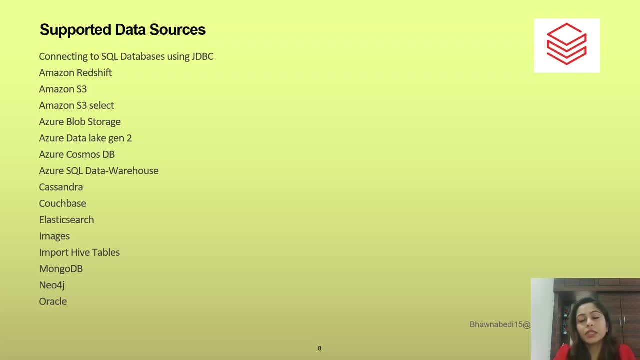 so when i say data sources, since you have databricks, right, and databricks is just a platform now to get the data and to send the data you need to, you need databricks to support the sources, right? so if you want to take the data from the sql server, 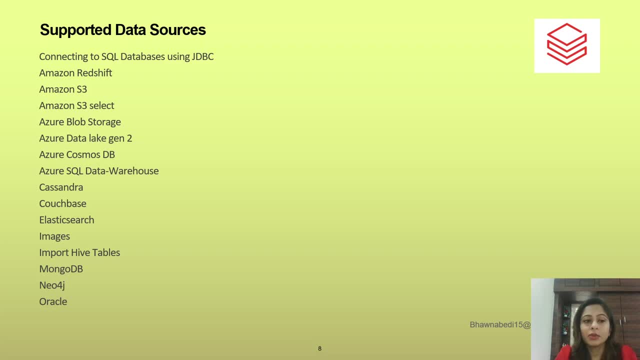 if you want to take the data from the sql database, right, not sql server. basically, sql database is the correct word. so if you want to take the data from the sql database, you want to take the data from amazon s3. you want to take the data from couchbase, you want? 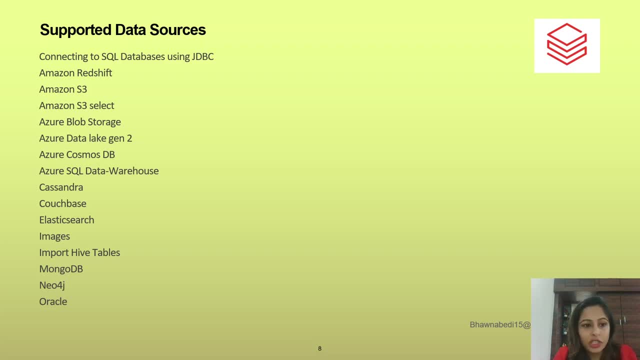 that databricks should support it. right and trust me, databricks supports a lot of these data sources, in fact i would say all of these data sources, what you can think of. on to the. you know the ppt that you see. you can connect to the sql databases using jdbc. we will 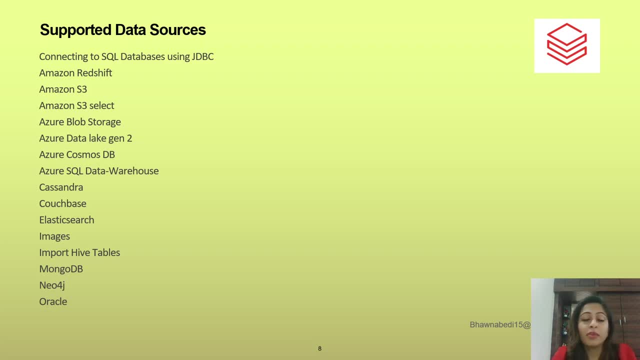 actually see how to. how do we do that? you can connect to amazon redshift. you can connect to s3. you can connect to, you know, your azure blob storage. you can connect to data like gen 2 cosmos db, which is your no sql database, basically your sql data warehouse. cassandra couch base. 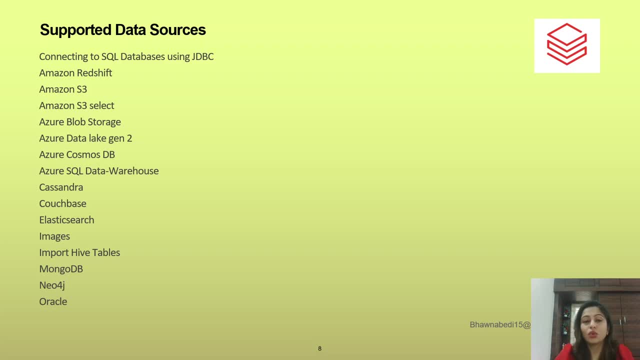 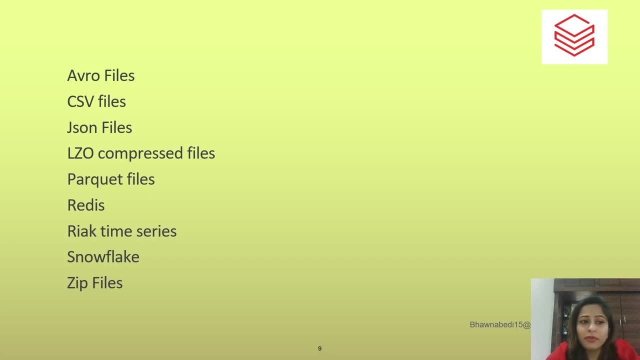 mongodb, you know oracle, you have all these sources and in fact, even you know many more. so, even if you want to, you know, bring in some abro files, json files, parquet files, redis cache, snowflake data warehouse, all these, you know file formats, all these file sources are actually. 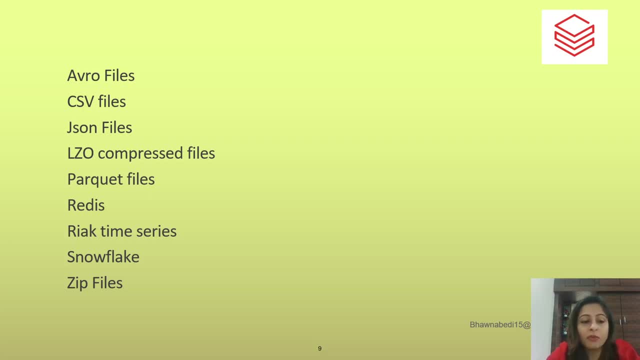 very well supported by databricks. we are going to go through all of them, almost one by one, in one or the other video for sure. so thank you so much. i hope you liked this video where where i just tried to explain in the layman terms what exactly databricks is, and you know what it. 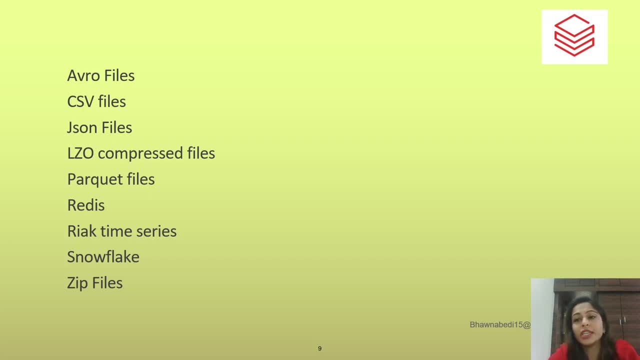 can do to a bit and we will cover most of the content in the upcoming videos. so thank you so much for being till here and do remember to like, share and subscribe to my channel.